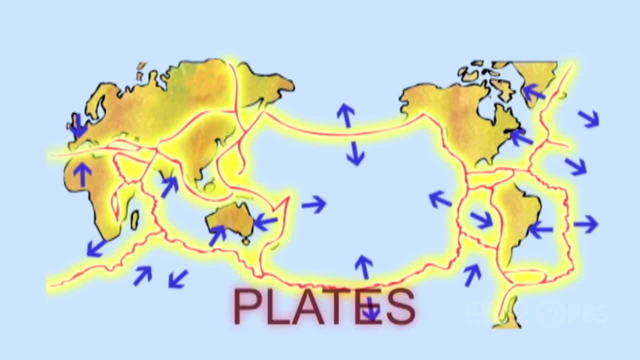 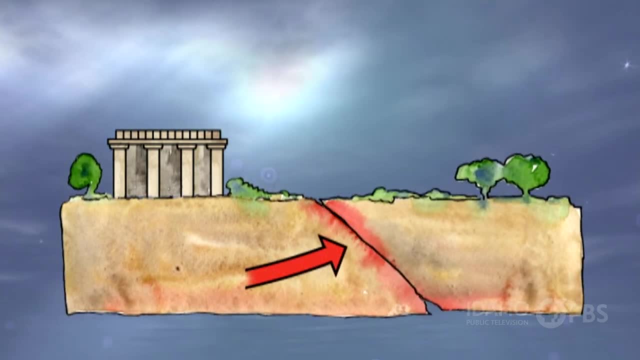 These plates are moving, sliding past one another, folding underneath or butting up against each other. When the pressure between two plates builds up to more than the rocks around them can stand, the plates crack and the energy is released in what we know as an earthquake. 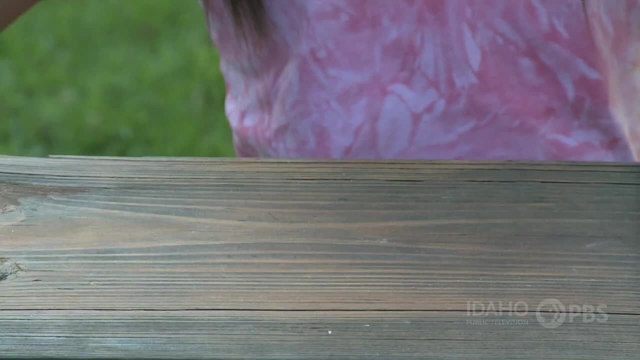 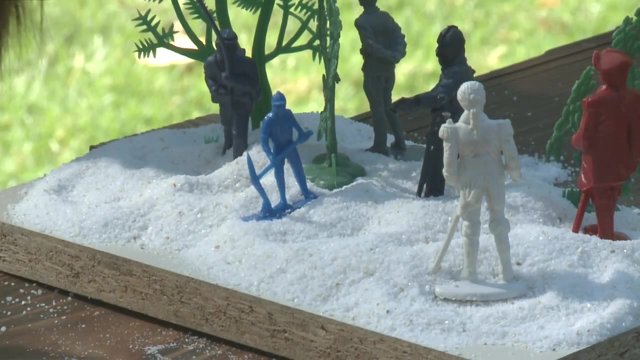 You can see why an earthquake can cause a lot of damage. Put two wood blocks together and cover them with a layer of sand, Put a few buildings and animals on top and then move one of the blocks, And that's what an earthquake looks like. 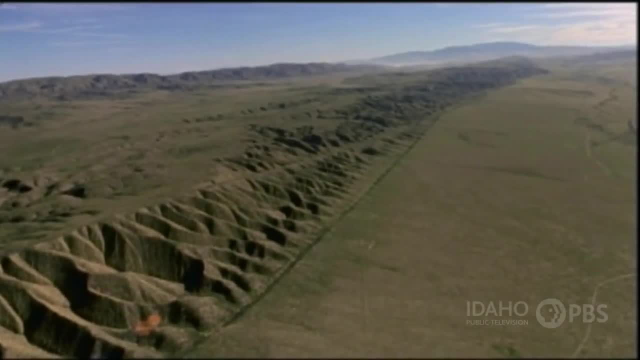 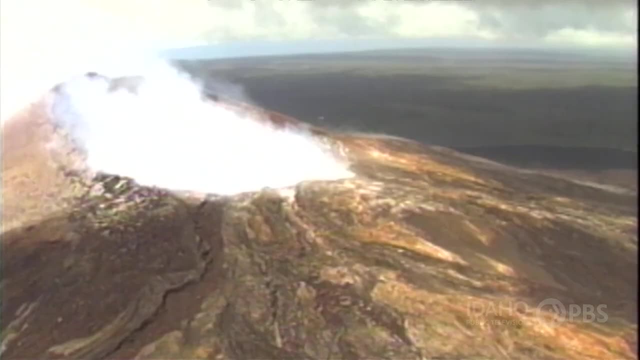 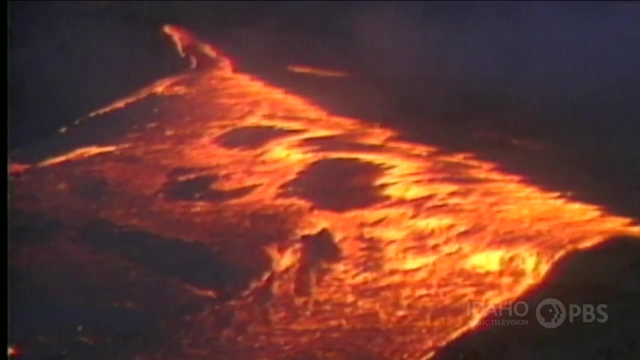 Earthquakes are most common where the plates meet. That's known as a fault line, And Idaho is number six on the list of states with the most earthquakes. A volcano is basically a hole in the Earth's crust where lava comes out. Lava is hot molten rock. 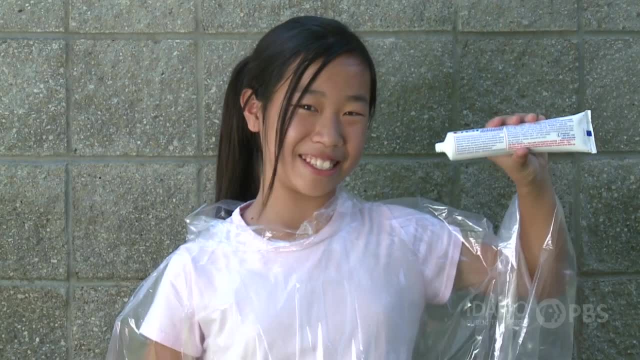 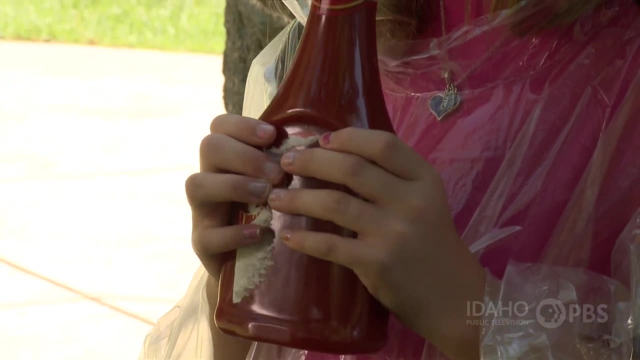 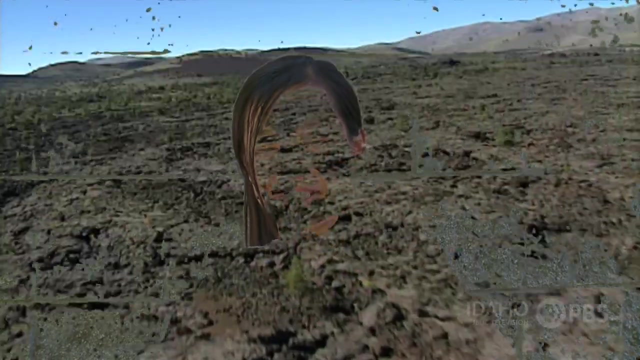 Lava has viscosity. Some lava, like this toothpaste, comes out thick. Other lava, like this ketchup, comes out like a liquid. Eventually the lava cools into rock. Ancient volcanoes created the twisted landscape you see at Craters of the Moon National Monument. 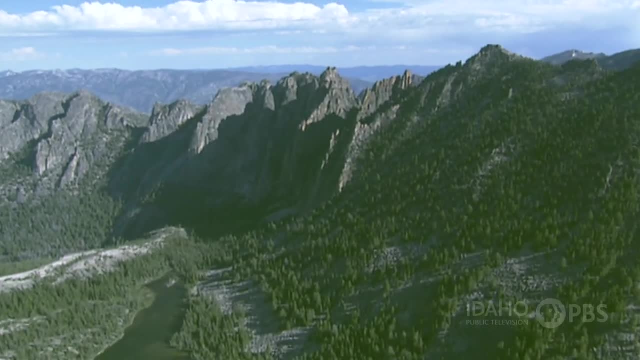 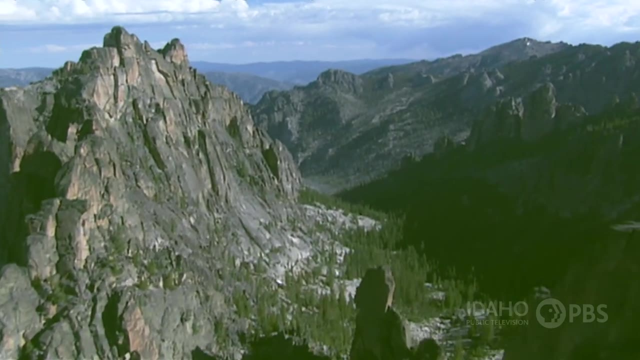 In some parts of Idaho the mountains were formed when magma or hot lava- still underground- pushed upward but didn't break the surface. That's called a batholith. These mountains are part of the Earth. They're called the Idaho batholith. 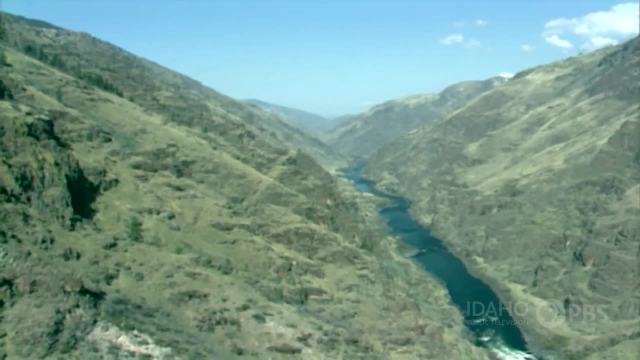 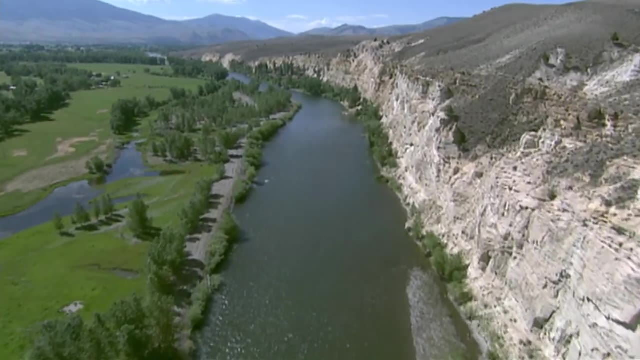 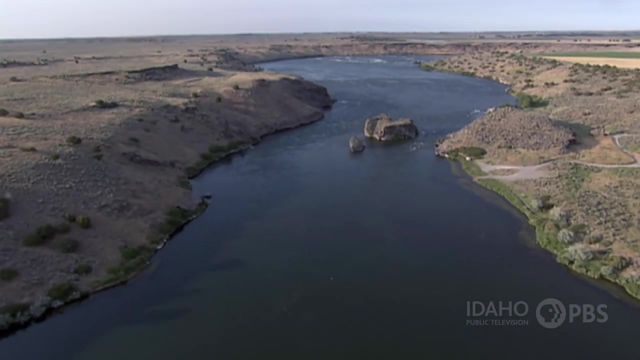 A little bit of water can completely change a landscape. Over time, moving water eats away at rock. So thousands of years later, what was a plain can become a valley. A flood can dramatically change the landscape. Fifteen thousand years ago, the Bonneville Flood scoured out the Snake River Plain, carving 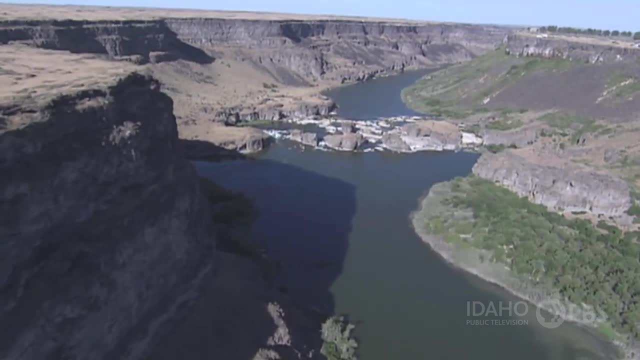 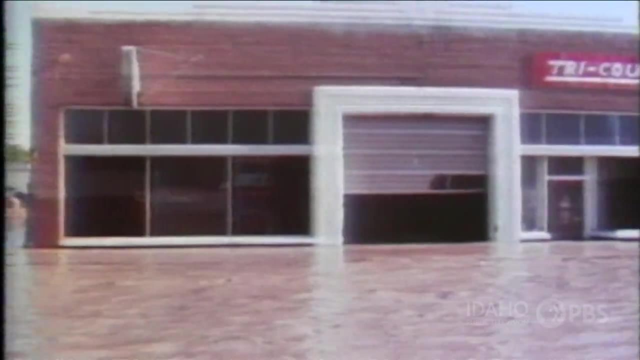 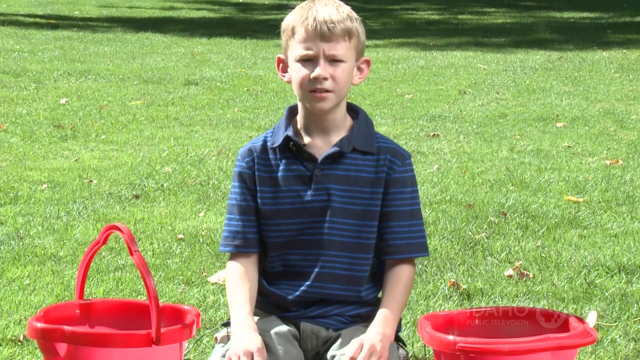 out the canyons at Twin Falls, And not all floods are caused by nature. When the Teton Dam broke in 1976, a wall of water almost wiped out many small towns, including much of Rexburg. How fast the water can erode the land depends on how fast the water is flowing. 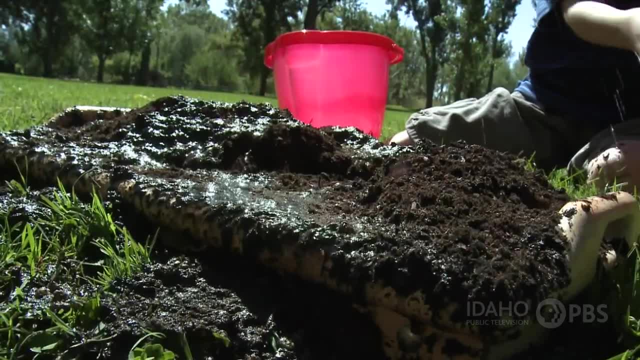 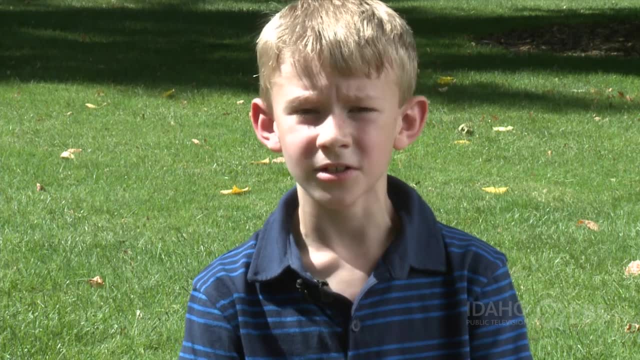 A gentle flow doesn't have much energy, but a flood has lots of energy, So the amount of damage to the land depends upon how much energy or force is involved. Glaciers are rivers of ice that carve their way through the land. The water flows through the canyons.